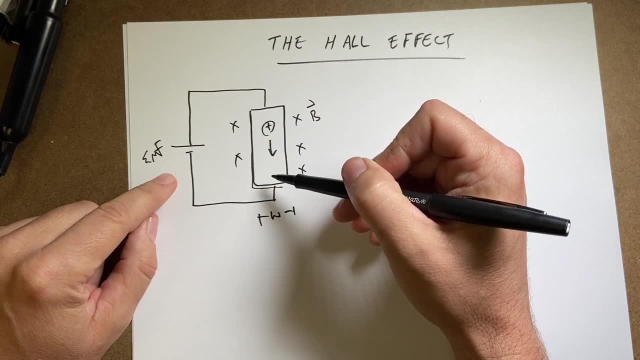 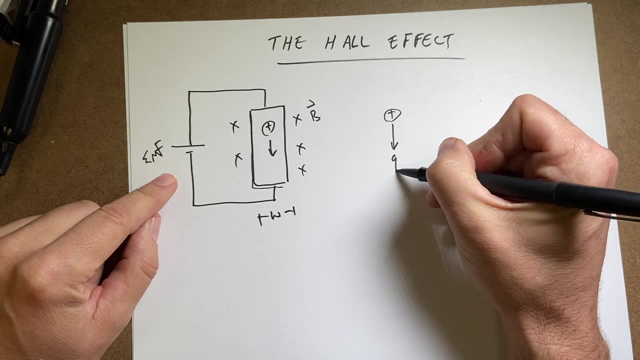 moving through there and they're positive charges moving in the direction of current. Well, what's going to happen to that charge? If I draw just that charge, I have QV. this way I have B going into the board, So then I can pull out my little, my little thingy. 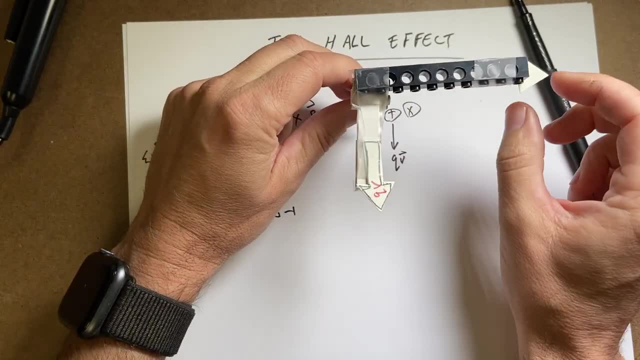 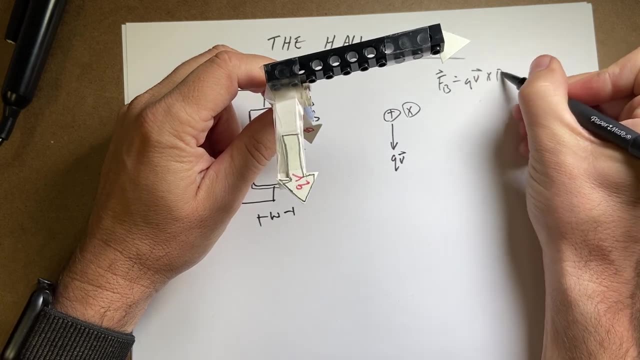 here QV like that, B is That way. so there's a magnetic force on there. FB equals QV, cross B And the direction of that's going to be to the right. So what's going to happen over time is that my metal. 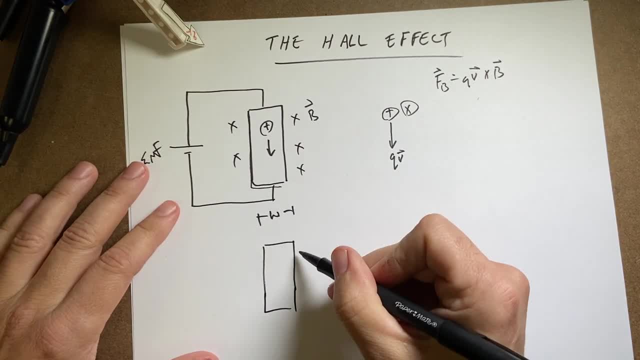 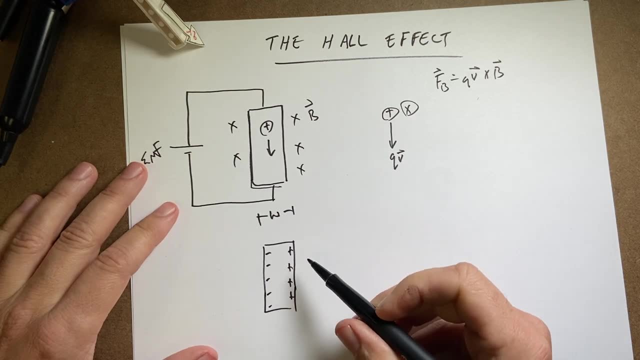 is going to look like this: I'm going to get positive charges on this side. They're pushed over here And that's going to leave negative charges over there. Now there's going to be an electric field inside going that way, So I'm going to have two forces on this. I'm 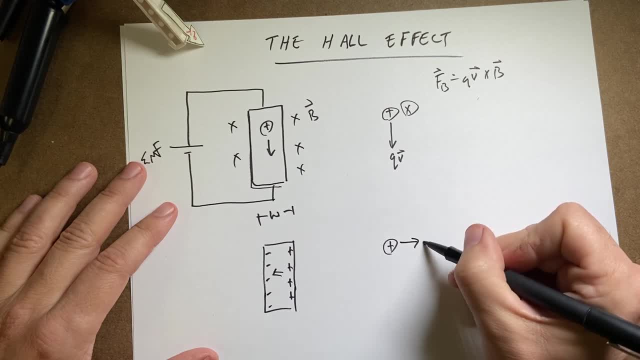 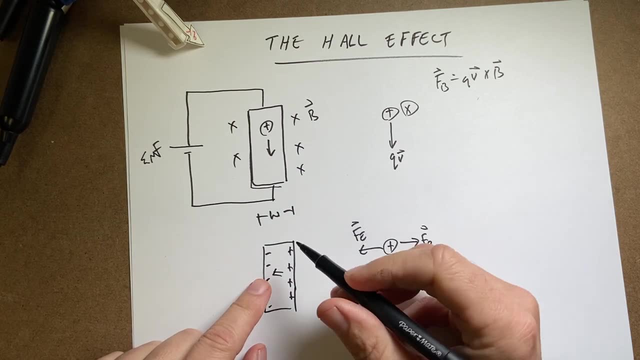 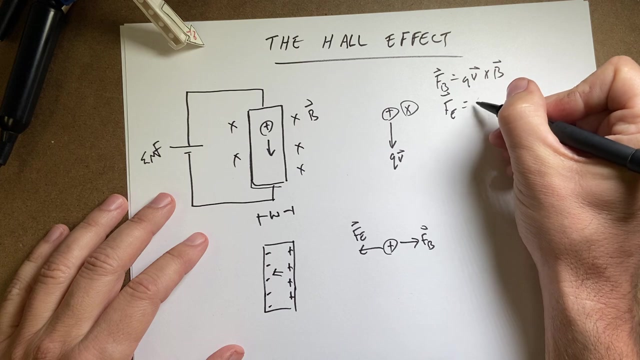 going to have the Magnetic force pushing this way, FB, And the electric force pushing this way, FE, And those that will continue to happen to have charges build up over here until those two forces are the same. So the electric force FE, is Q times E, So everything's perpendicular. 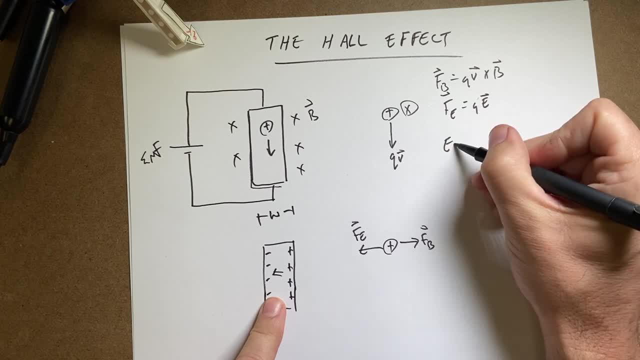 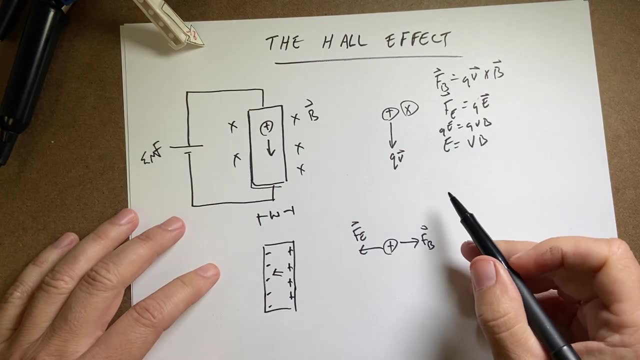 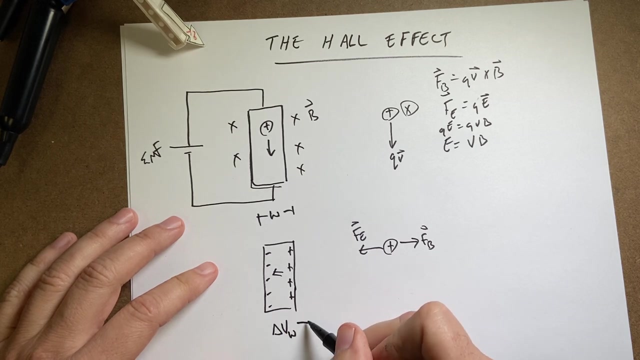 here. So this is going to keep happening until E equals VB. Technically it'd be QE equals QVB, but the Q's cancel. Now one other thing. I can find the change in potential. I'll call that delta VW because it's about the width. I can just measure that And I'll use that later, But by measuring 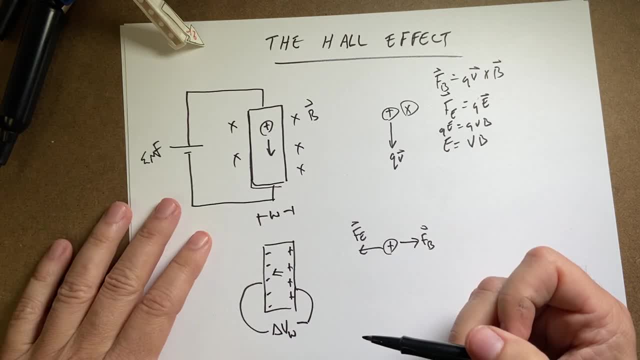 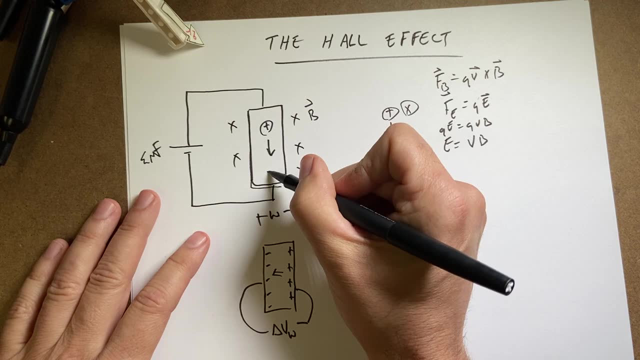 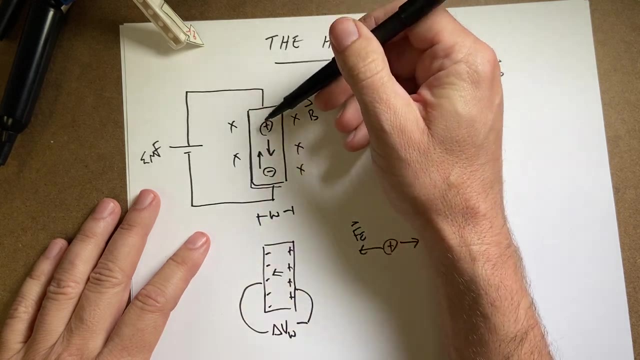 that I actually could tell if this is positive charge on the left or negative charge on the left. Okay, Now suppose I don't have positive charges, Suppose I have negative moving charges, And so for the same circuit these negative charges would be moving that way to make the electric. 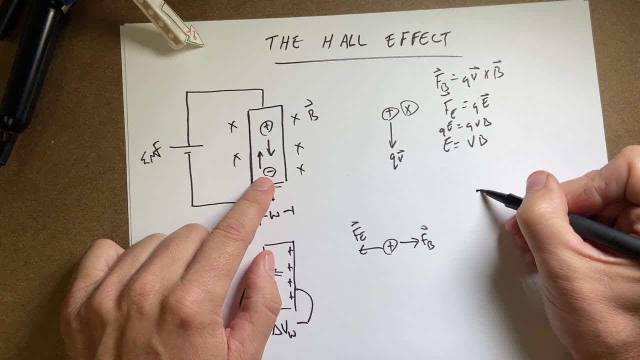 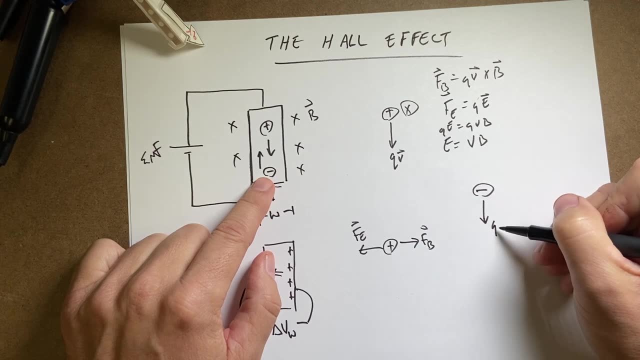 current. going this way, What's going to change? Well, let's draw my forces. So here's my negative charge. Here is: QV is down to the right. still, Even though V is up, Q is negative. So QV is that way. 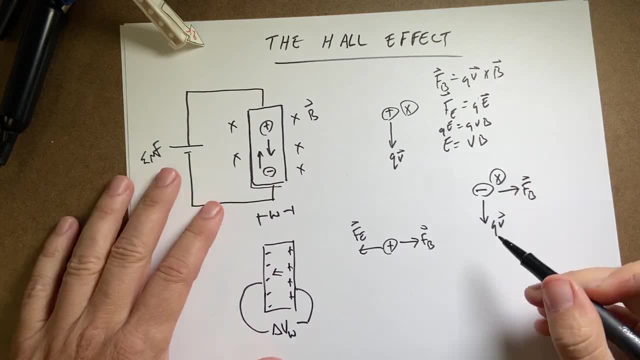 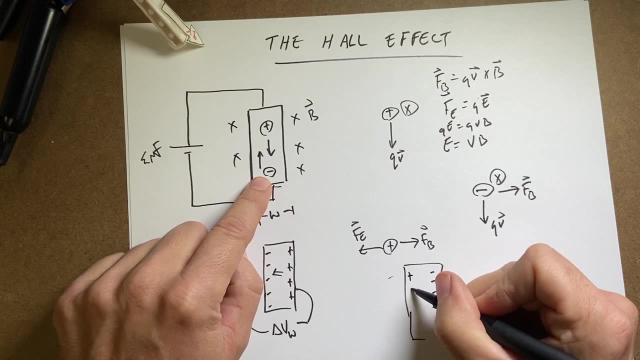 B is into the board. FB is that way. So now, in this case, I'm going to get: the magnetic force is to the right, I'm going to get negative charges on the right and positive charges on the left, And I would get a different. 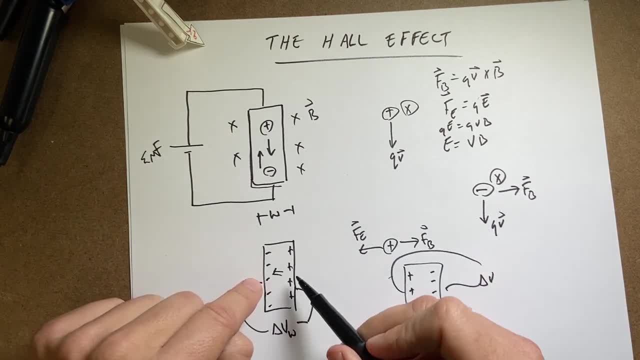 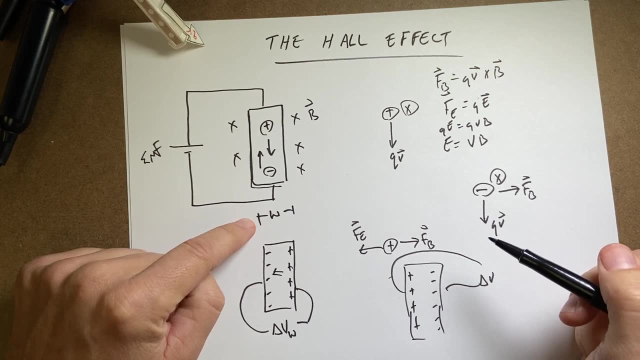 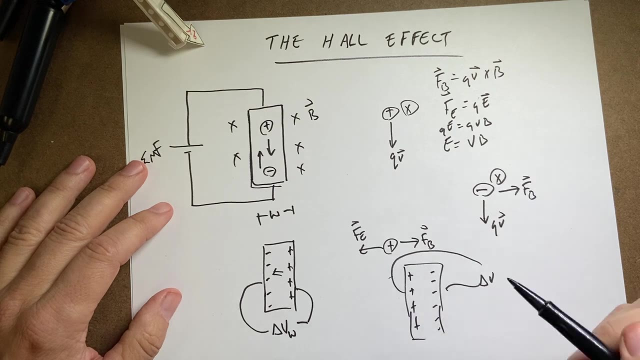 Delta V. So by measuring this perpendicular voltage, through this I can determine whether the mobile charge carriers are positive or negative. In most cases we see that moving charges doesn't matter if you have positive charges moving down or negative charges moving up, But in this case it does. So you can actually detect that change in voltage. Now 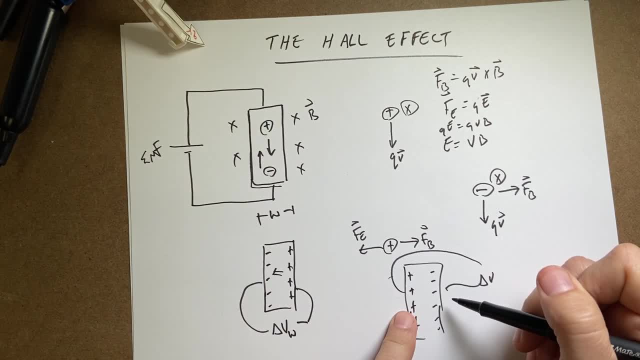 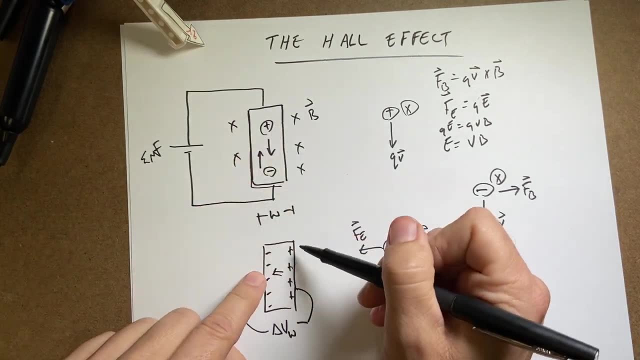 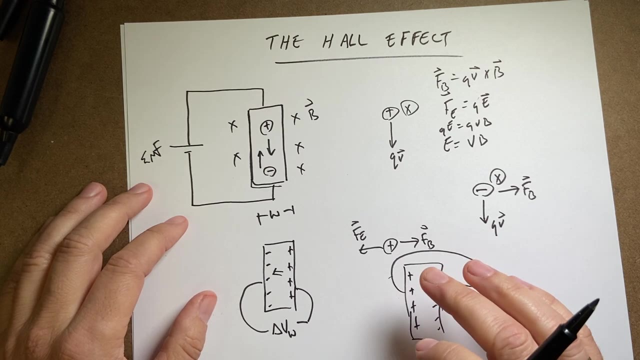 warning: this is a very, very small voltage difference here, So you need a really good measurement tool to determine that. But that is the Hall Effect, this side potential build up due to a magnetic field. But wait, what if I do this backwards? What if I don't know the value of the magnetic field I can? 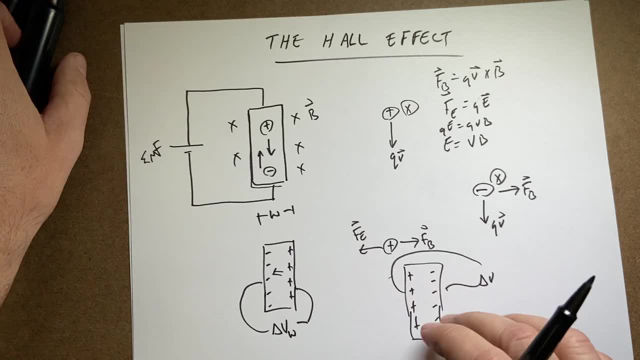 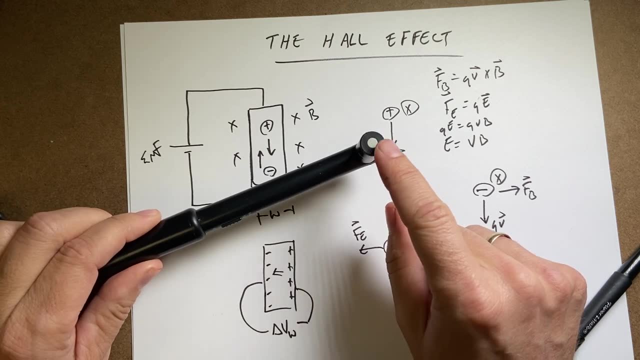 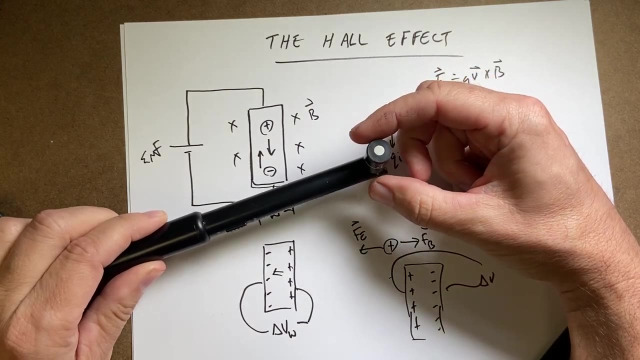 use this to calculate that. So this is a Hall Effect probe. in fact, I'm not going to draw the picture. This is a small piece of sensor up here with an electric current that runs through it. you measure the perpendicular voltage on that to determine the value of the magnetic field. 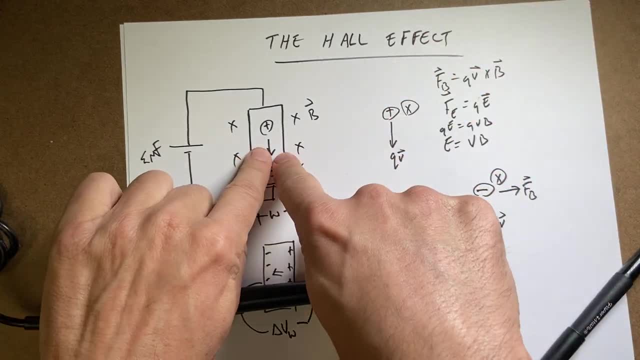 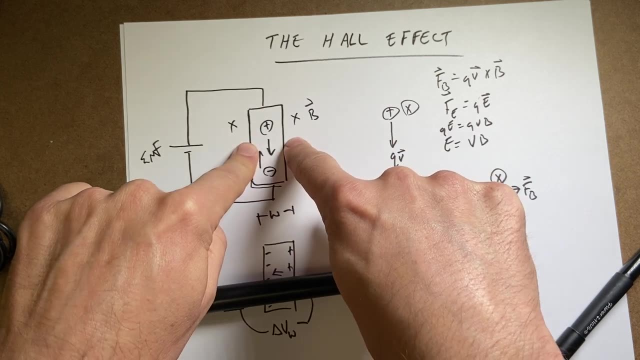 you have to know the width of the thing and you know, need to know some things about the drift velocity and the current and all that stuff. but what you do is you put this sensor in the magnetic field. a voltage builds up on the side, just like this, and you measure that voltage and once you 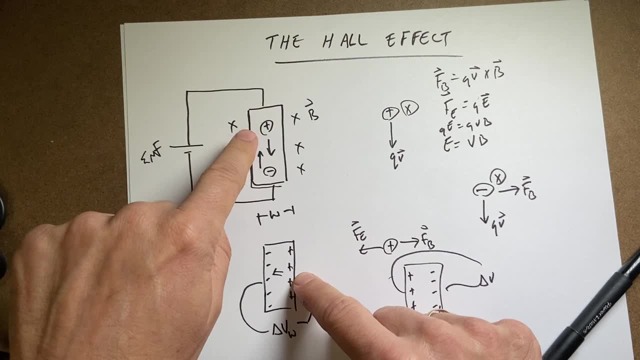 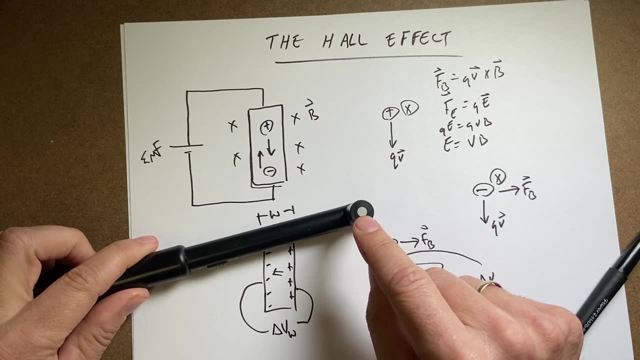 know that voltage, you can then go back. if i know the value of the current and the drift velocity and the charge carriers and the width of the sensor and all that stuff, i could calculate the magnetic field. your phone detects a magnetic field and it uses that to as a compass, so it 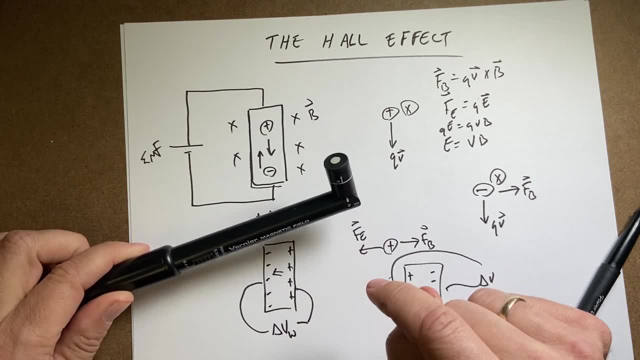 has one of those in there too, but it's a very, very small magnetic field detector and it works pretty well and it's all based on the hall effect.